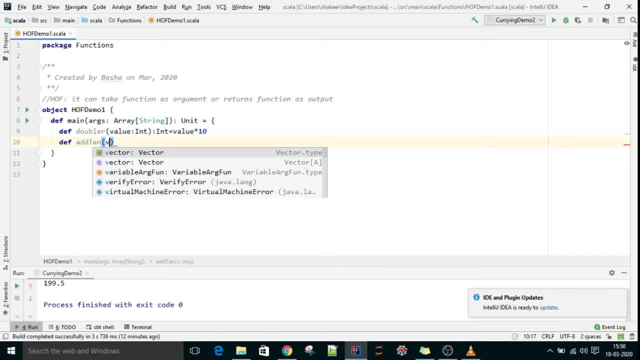 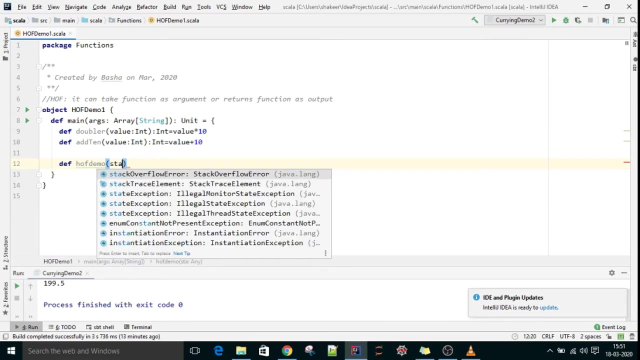 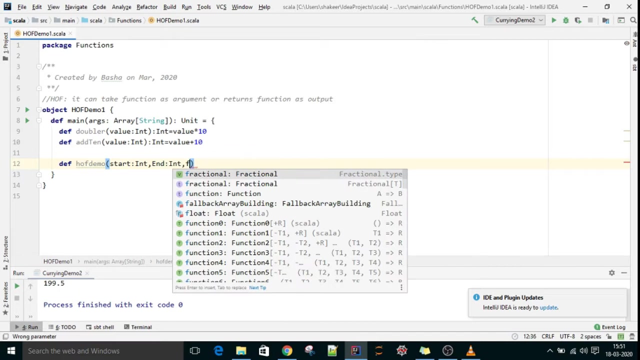 So okay, value, same value into type. Okay, return type, int. okay, value, plus done. I have created two functions for methods. Okay, so here def, HOF demo. more okay, some start start parameter into end parameter, into okay, here some F, okay, colon integer, here it written it. we have to mention here any, well, any. 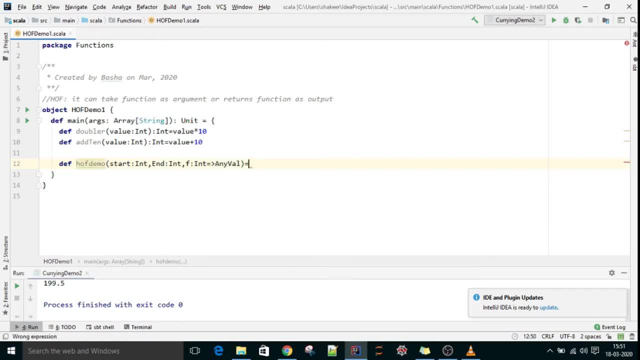 well, okay, so I have created doubler one function. what it is doing that, whatever element parameter were passing, it is multiplying with a 10. here I add 10 method. what it is doing: whatever parameter were passing, it is adding 10. okay, so this is a higher, higher adder function. hif demo: it is. 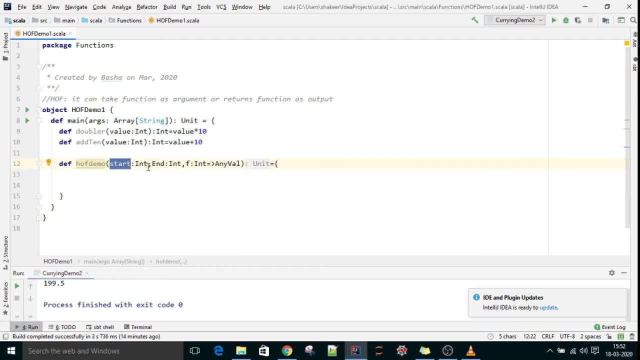 first one, first parameter. second parameter: okay, third parameter is a function, okay, it is. so we are passing it is hif, demo is a function and we are passing one more function as a input treat. so so what we can do, is I okay for loop without the start range and end range, start value and start to. 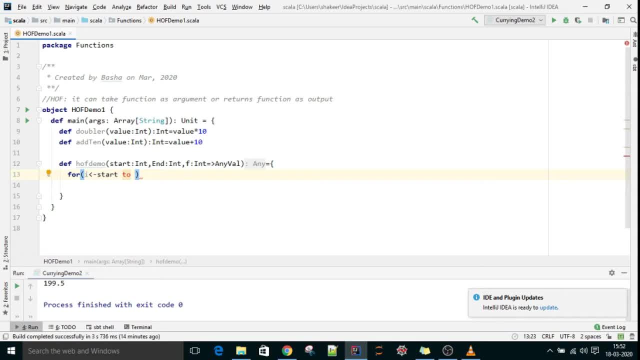 end you, you end, okay, print Ellen some F of I. okay, so this is a higher adder function. we are, we are calling here: print Ellen H for F, demo of start range. to end the range: 10. okay, yeah, can you, you, you, Okay, good bye. So what we are doing is we are calling two functions here: double return, third method. we are passing third method. we are creating as a third parameter for this third method, we are passing another function. 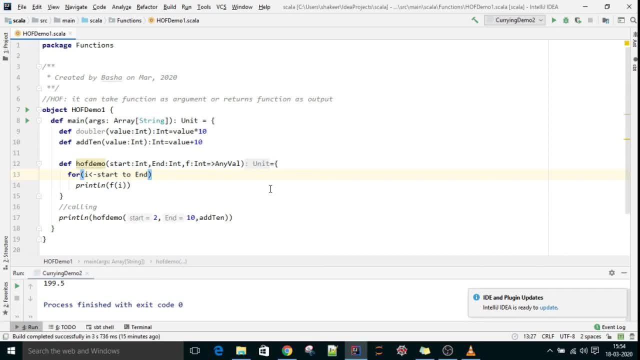 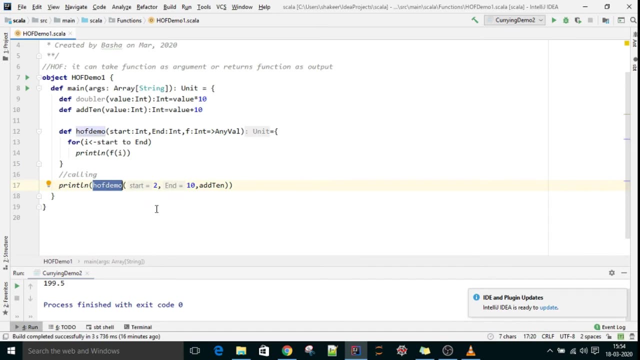 So this will become higher order function because it is taking one more function as a input and returning function. So here, println, I am calling this higher order method. So these are the two variables, but this one is a function. We are passing function to a function as argument. 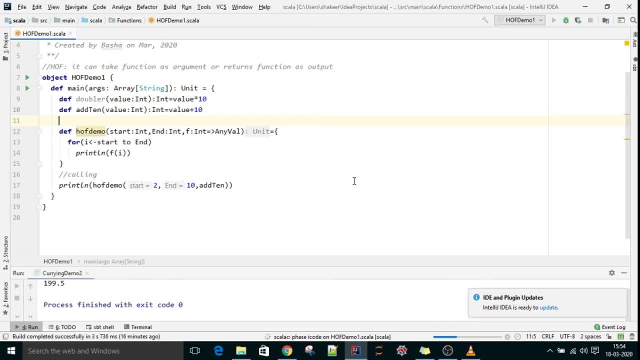 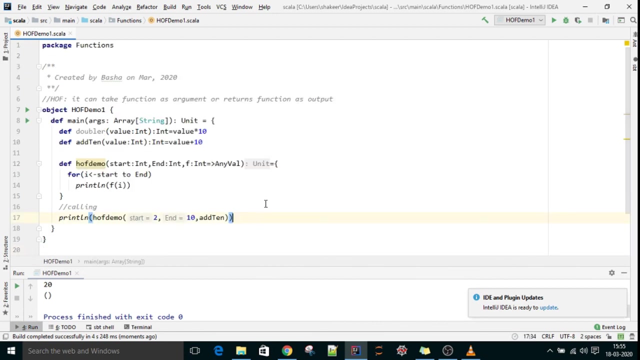 So 2 to 10, here 10,, here 10 means 2, 2 plus 10,, 12, like that 13,, 14,, 15,, 16,, 20.. So this is called higher order function. Thanks for watching this video.